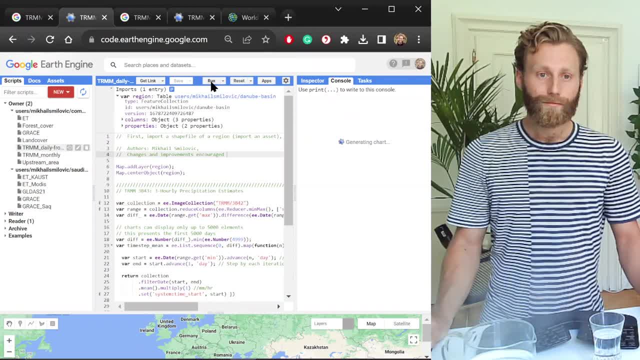 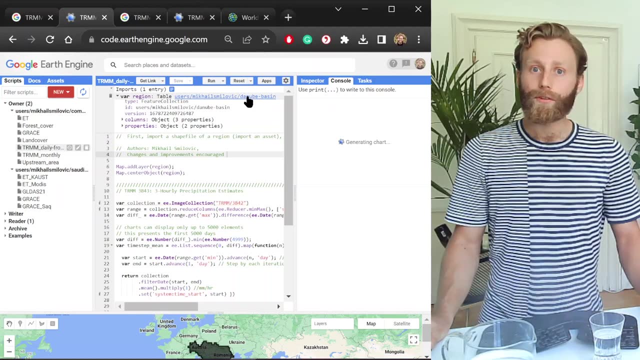 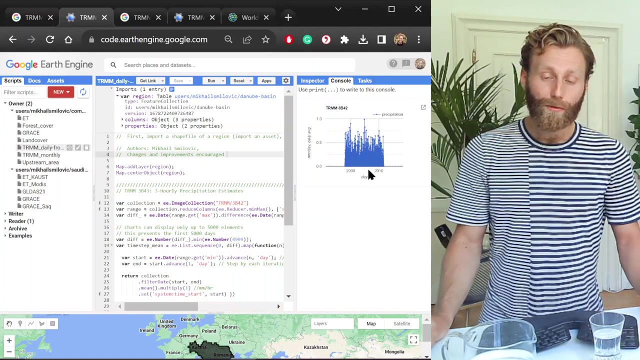 If we push run right now we're looking at precipitation averaged over the Danube Basin in Europe. The script is generating the millimeters per second, The average millimeters per day- of precipitation for the period available. Let's open this up. so the script is finished running. 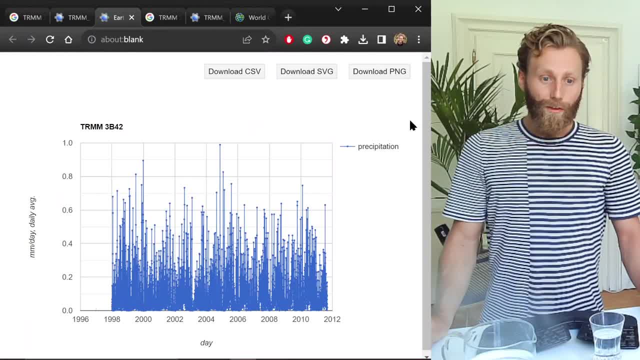 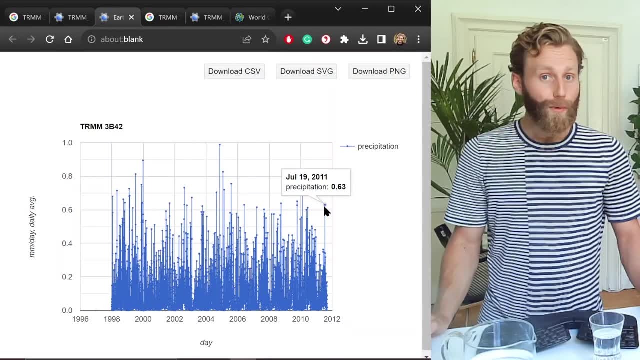 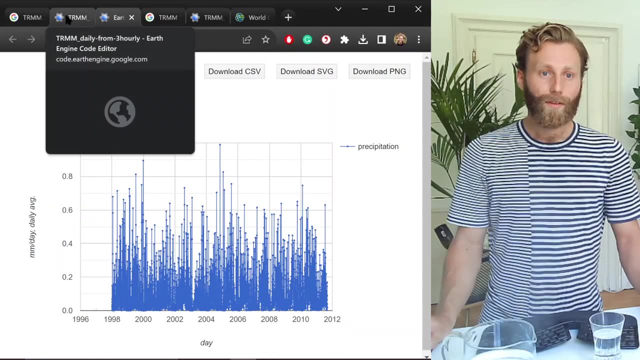 Let's use this pop-out window. We see, from around 1998 all the way to 2012, or midway through 2011,, the millimeters per day averaged over the Danube Basin. If we push on the second script link below, it will take us here: 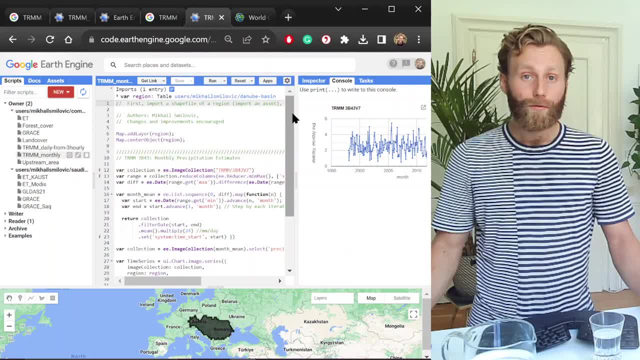 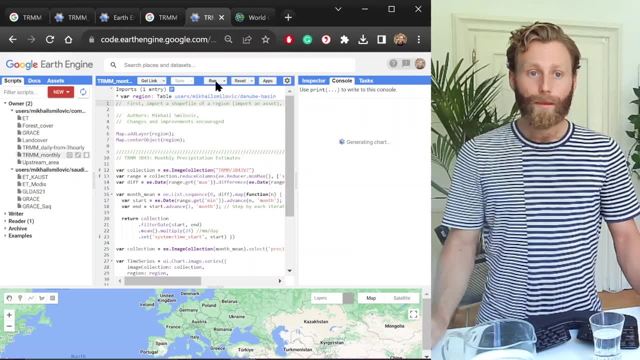 Perhaps this is more interesting. It will give us the monthly average millimeter per day for the area of interest, for the time series, If I push run again right away. the region that's going to be downloaded right away is the Danube Basin. 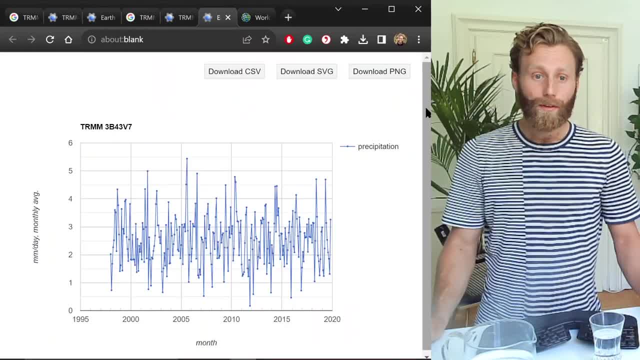 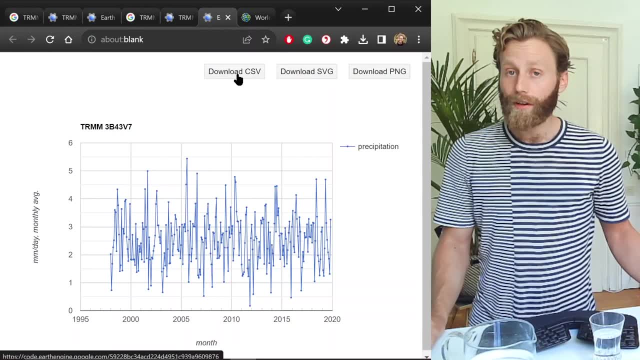 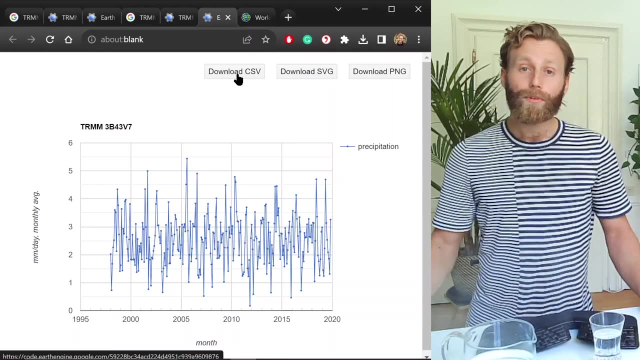 The script is finished running, We do the pop-out window. The pop-out window is nice because we can download the CSV, which allows us to open it up in Excel and do whatever analysis or further figures we're interested in. This is the millimeter per day average precipitation, that's rainfall and snowfall. 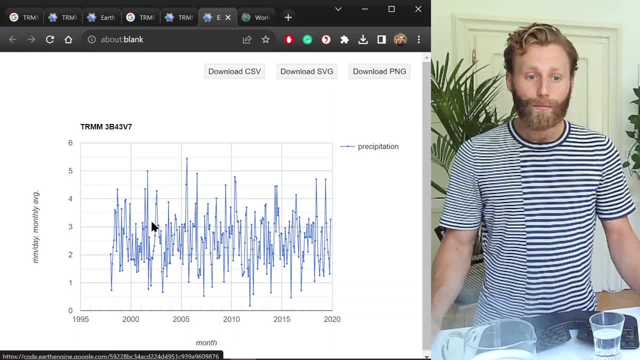 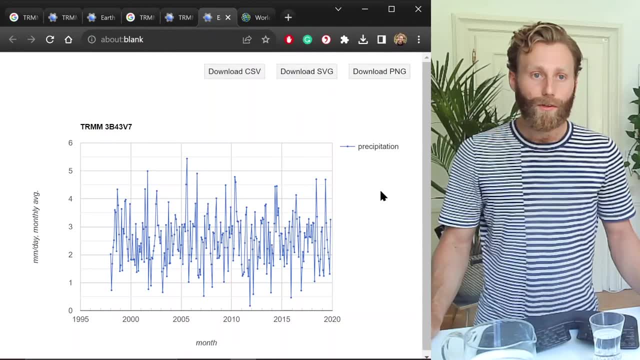 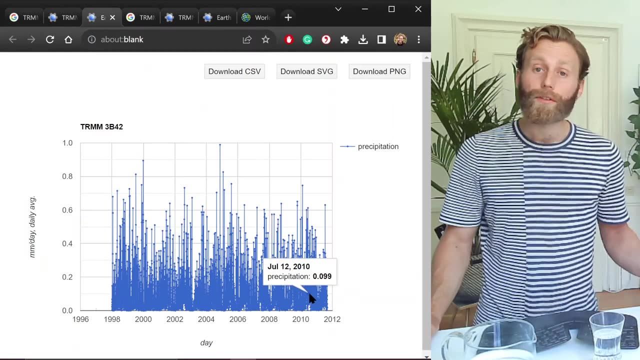 or liquid and solid precipitation from 1998 to, in this case, all the way up to 2019.. They have different dates of availability. This previous one, when we're looking at the daily, the three hourly turned into daily- 1998 to 2012,. 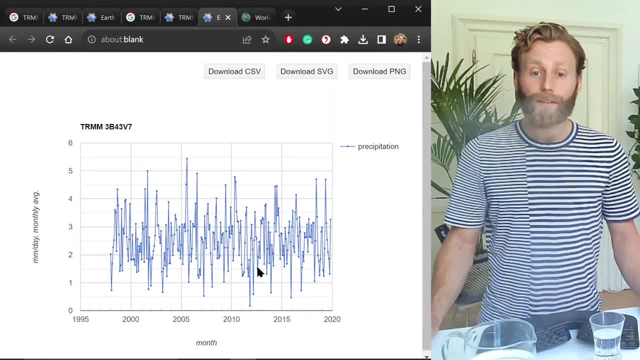 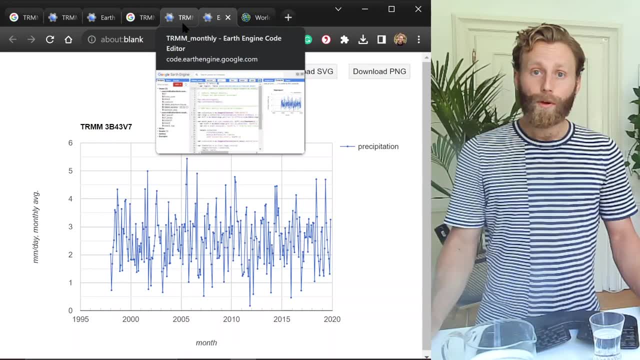 and the monthly we're going from about- yeah, also 1998 to 2020.. Now you may be interested in doing it for a region other than the Danube Basin. What you require is a shapefile. I will demonstrate this for the country of China. 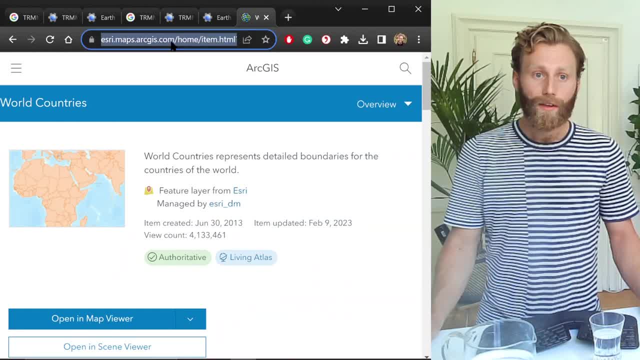 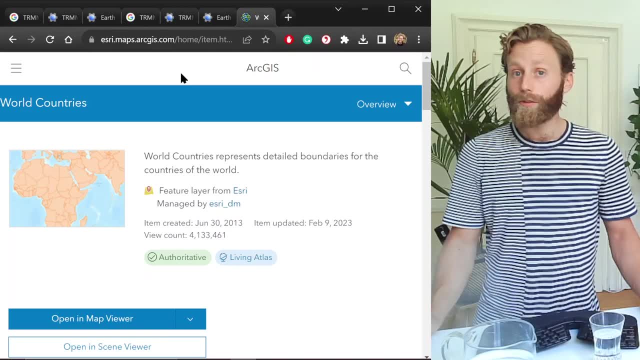 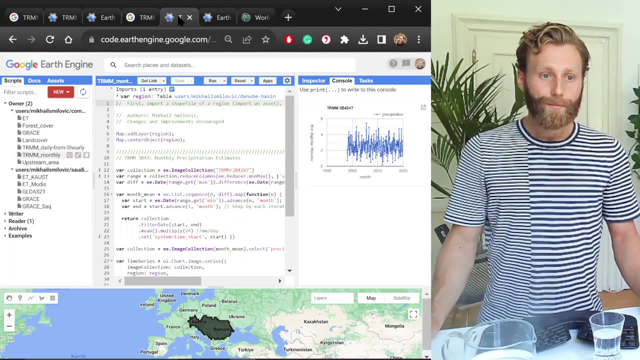 So I have come to this world country. some ArcGIS. I'll also include this link in the video description. Then, using ArcMap, I turned the country of China specifically into a shapefile and I will upload this now. So, going again, let's just do this for the monthly. 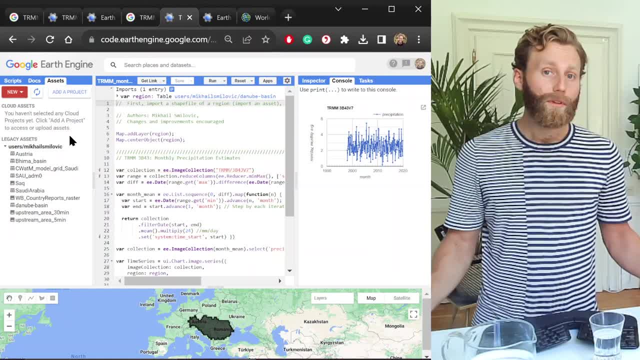 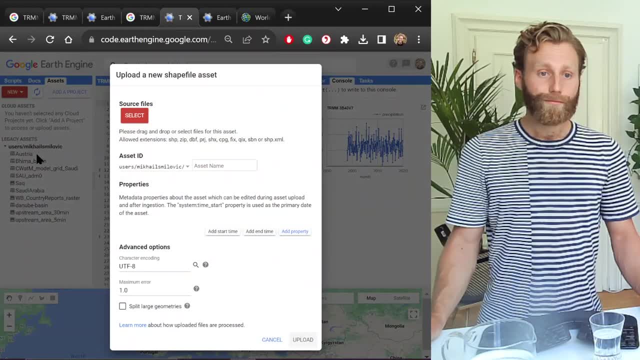 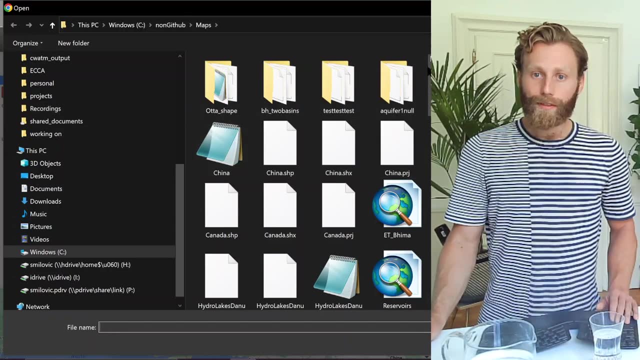 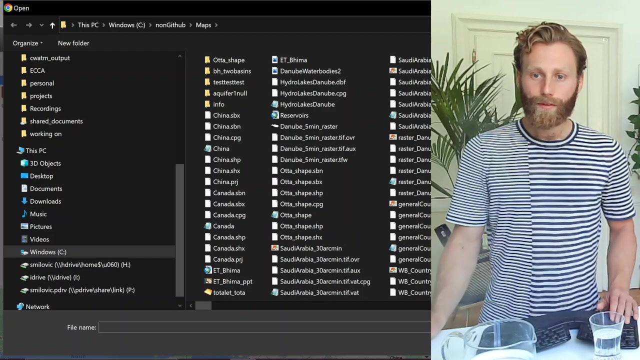 Let's go into assets and I'm going to upload the China shapefile that I have created. So I'll go to new shapefiles. select- I'm looking for the four files. Let's view this as a list And sort by date. 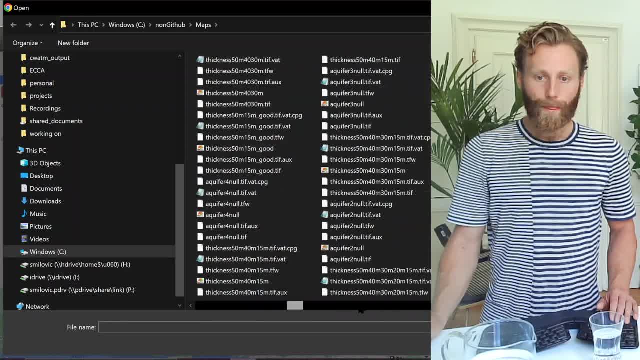 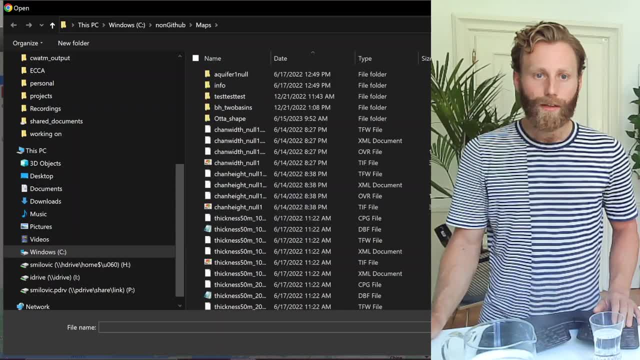 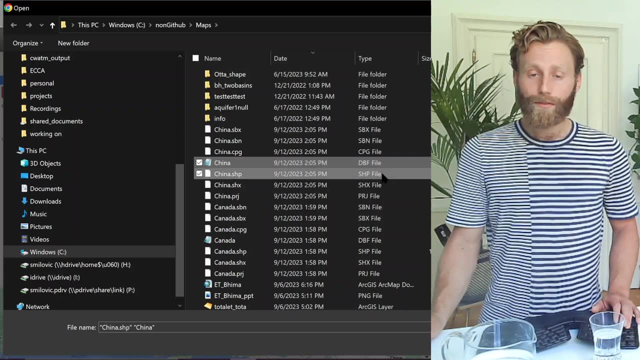 Okay, Okay, I'm looking for the files, Sort of one, of even different details. This is perfect, Just what I want. Okay, I'm looking for the DBF file, the SHP file, the SHX file and the PRJ file. 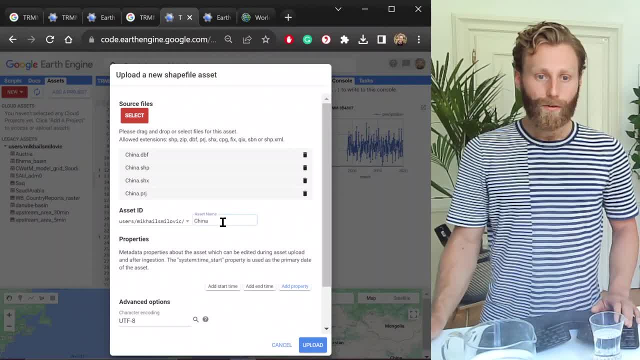 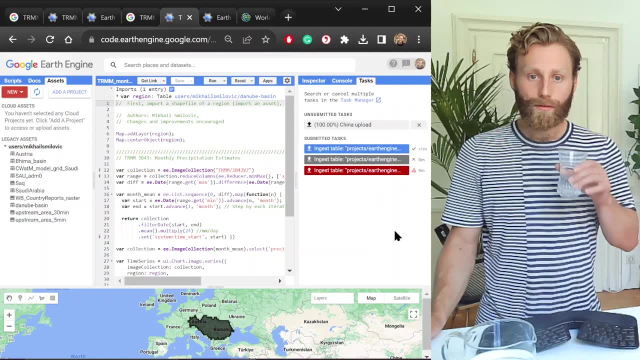 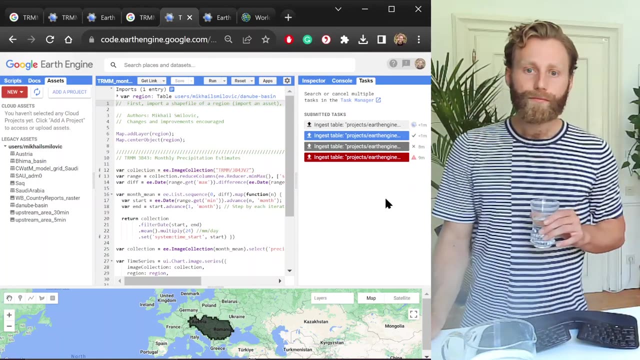 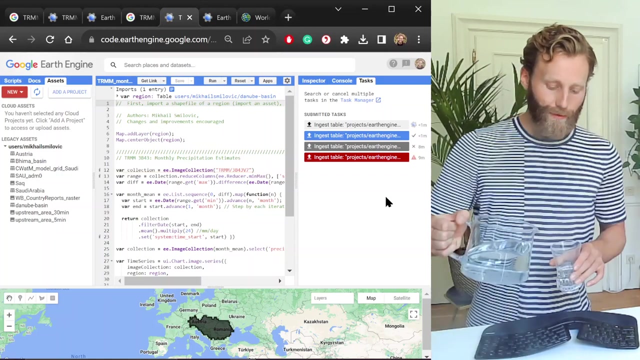 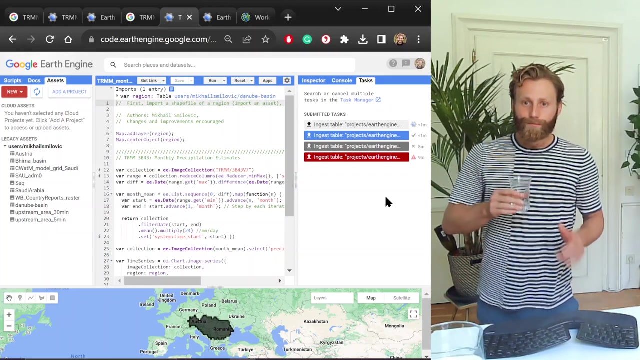 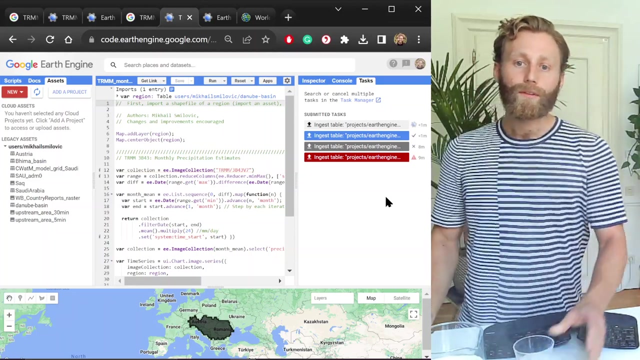 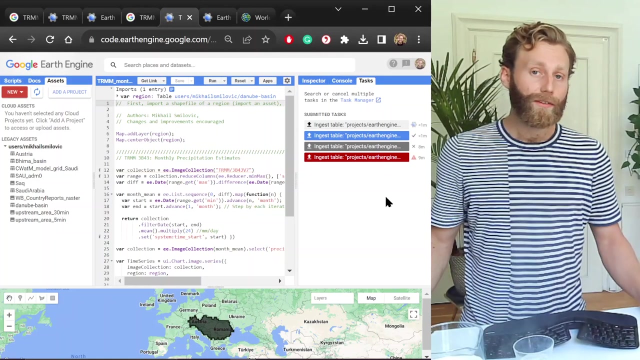 I'm going to upload these four And I'll call the asset name China. We see in tasks. we'll see that it's uploading, Already uploaded. That's fast. No, it's uploading now. Okay, I'm going to upload this. 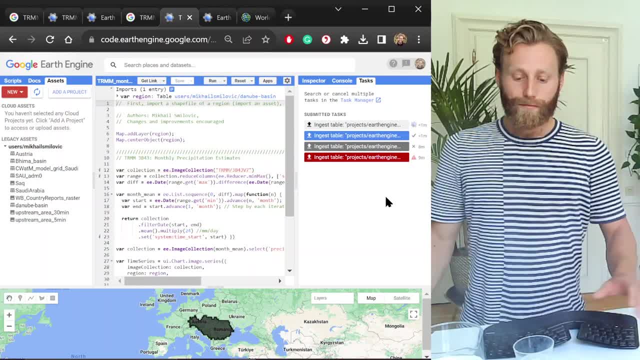 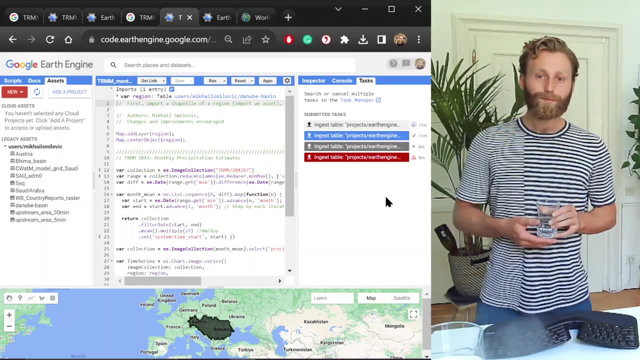 So, again, the first link is providing a daily average millimeter per day, and the second link is allowing us to look at monthly average millimeter per day. Okay, Okay, I'll wait until it runs so I can click on that. 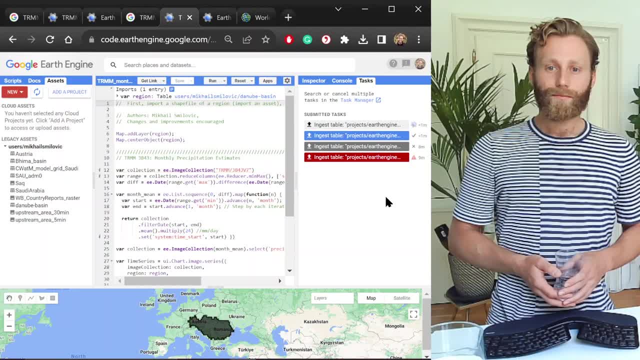 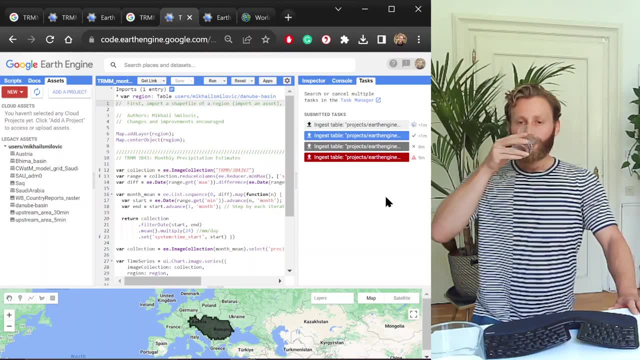 Okay, so now it's running, and you see it's already running and I'll wait for the new single to come up here. Okay doing that, And then we'll just wait for the new single to come in, and then we'll see how fast it takes. 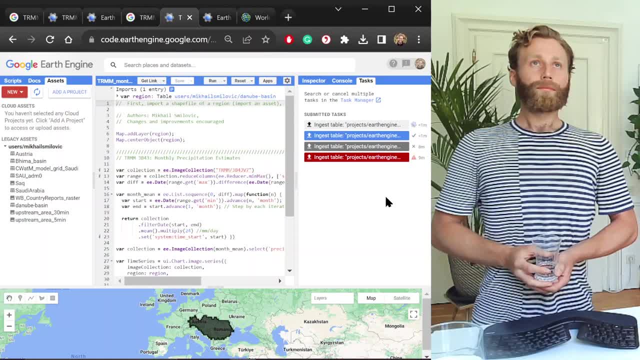 I've loaded all my files here, So I'm going to wait for it to run, and then I'm going to wait for it to run, and then I'm going to wait for it to shoot, and then I'm going to wait for it to run forever. 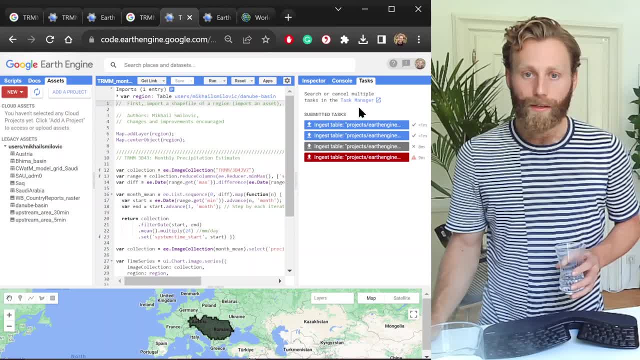 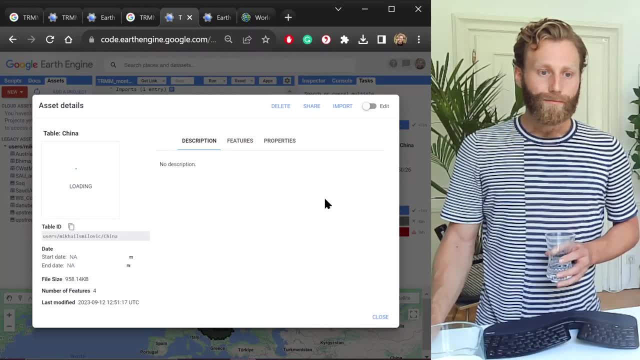 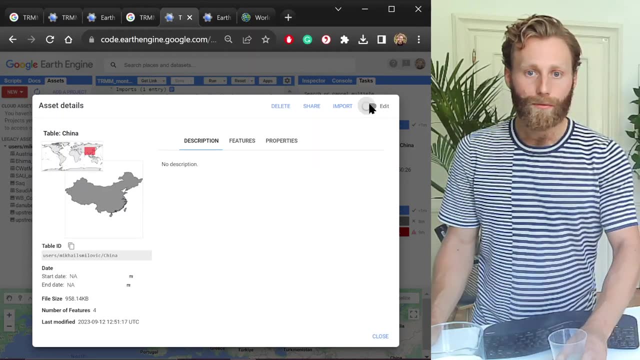 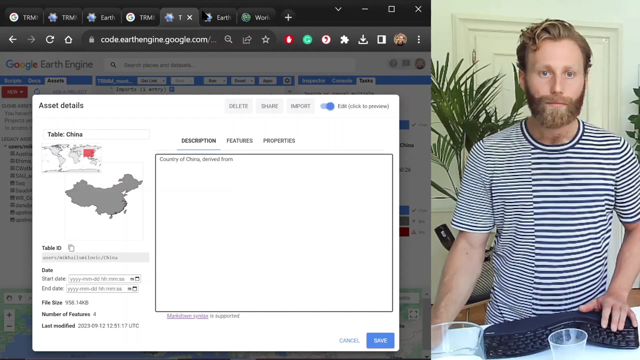 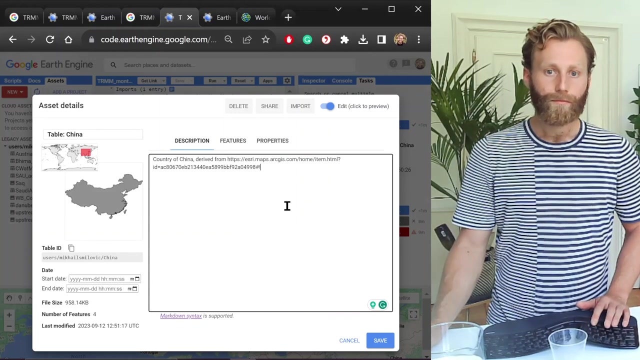 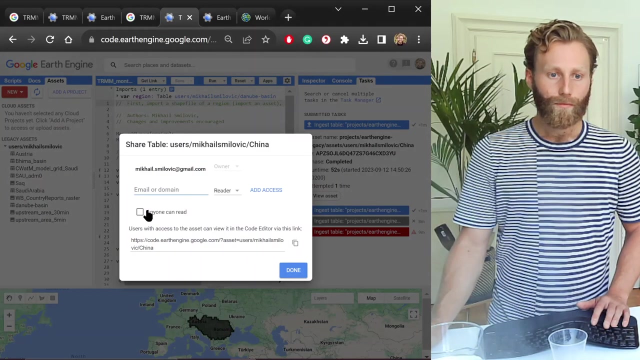 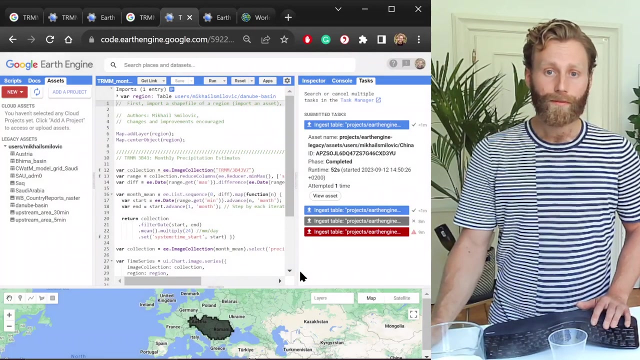 okay, clicking on our new asset, I can go view asset. we see here the country of China. let me just edit this and I can make it shareable. derived from: okay, so anyone can read. I'll also include the link to this China asset in the video description. okay, so we've got view asset and now let's go import. we can click import here. 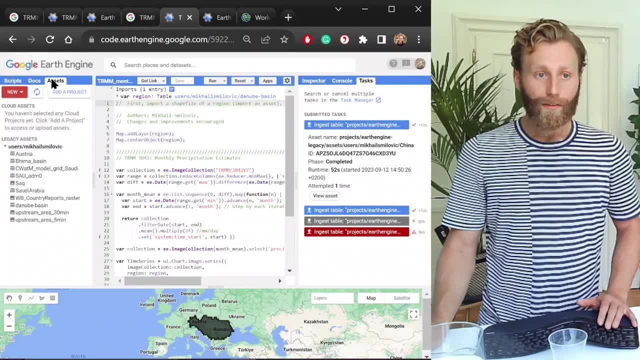 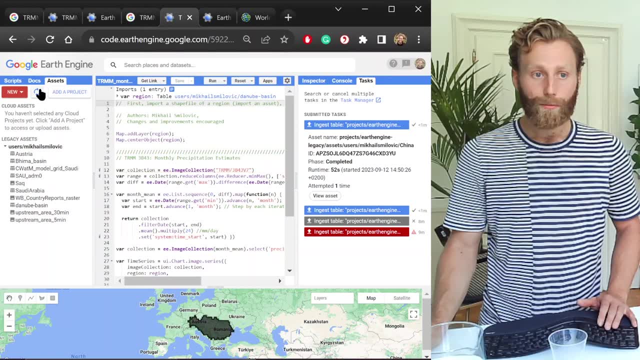 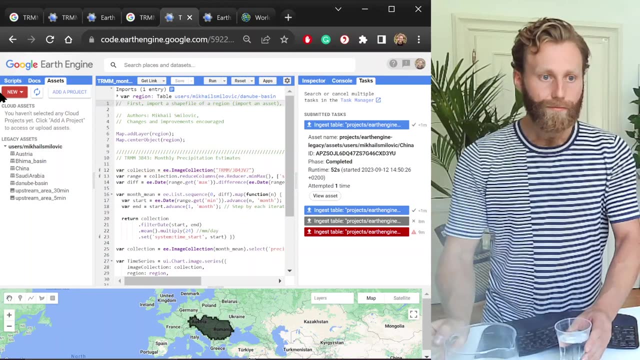 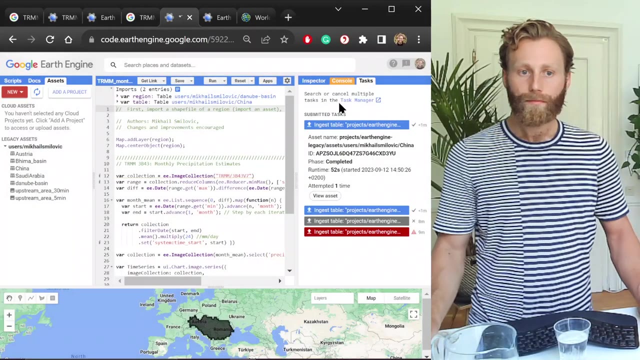 or we can go into assets again here. so let's go back to assets. China isn't yet here, but let me push the refresh button and then it's here. so I'll click China. yeah, it takes me here, and then we push import. now what we have. 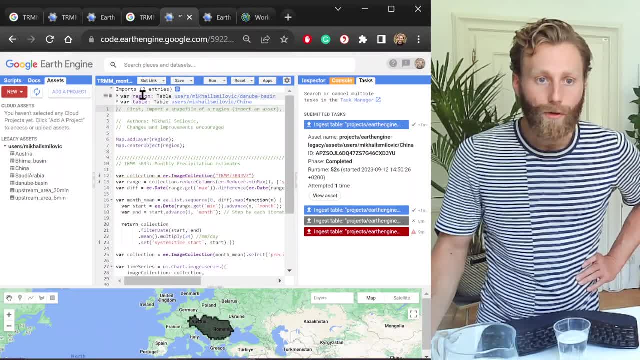 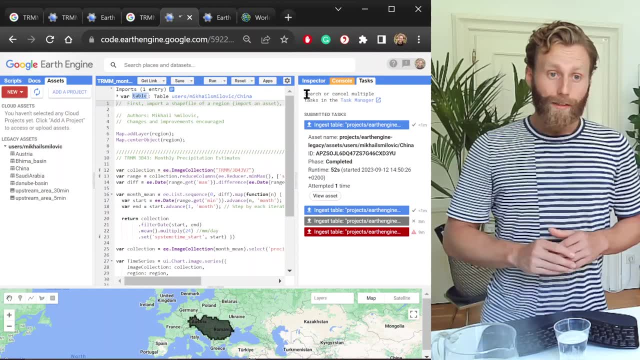 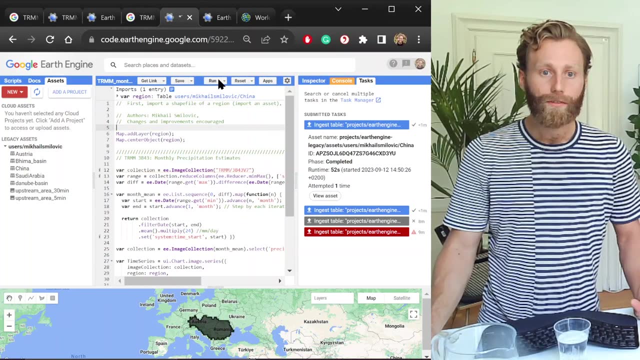 to do here, when you put your own region in, is delete the old one. see, it was called a region. delete this and the imported one is called automatically table. let's rename this to region region r-e-g-i-o-n and click anywhere. now let's run the script. I am in the second script, that's. 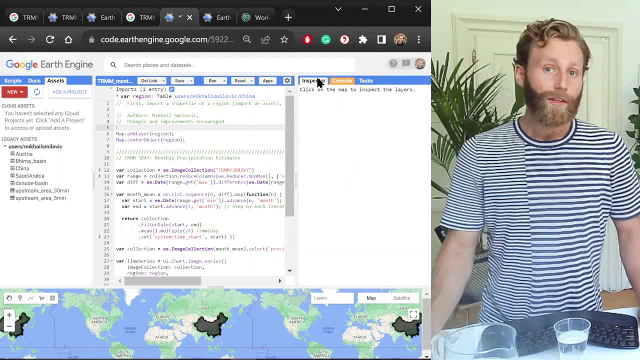 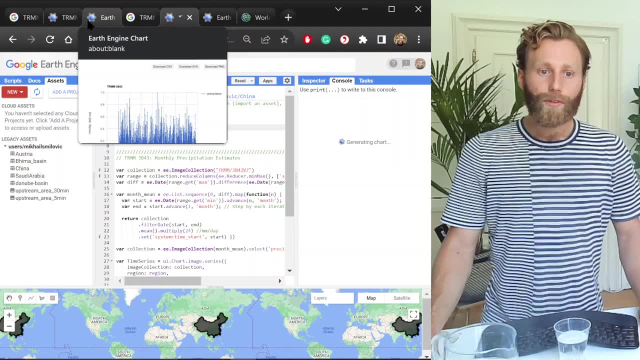 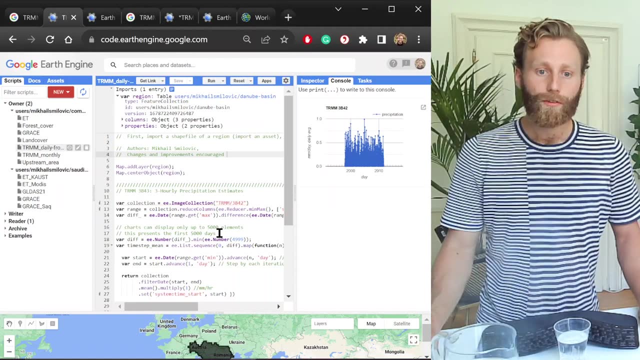 showing us the monthly average millimeter per day. this will also work in the daily. let's go to console. it's generating the chart. something interesting about the first daily: it only allows us to see 5 000 points in the time series. so we're actually, you see, here it's. 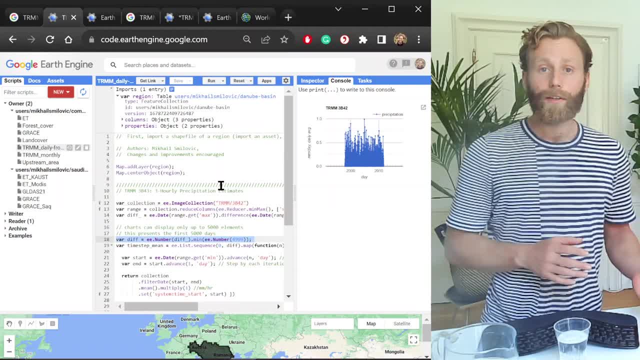 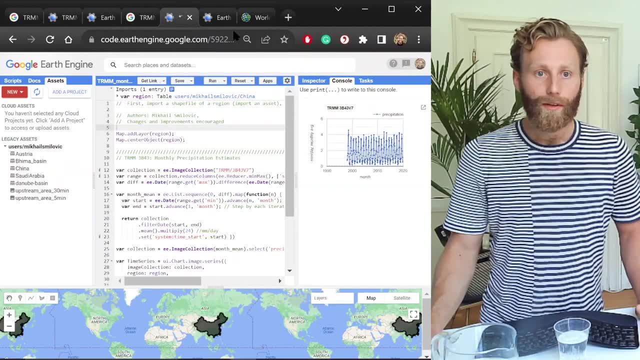 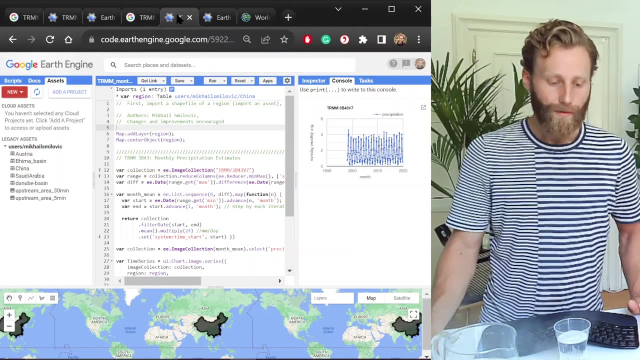 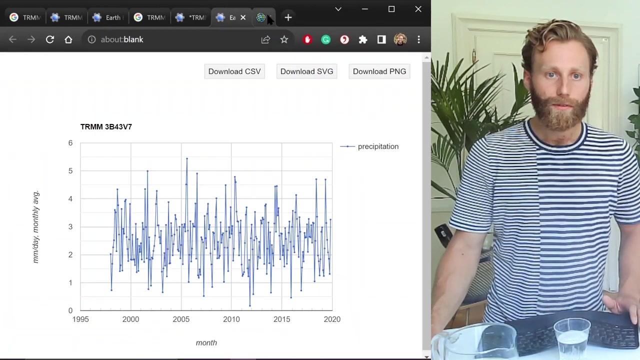 limiting the data to just the first available day, to 5 000 time steps after that for the monthly. okay, great, actually, because this looks so different than the Danube, I'm going to. okay, let's, I want to compare the Danube and China and close these links.